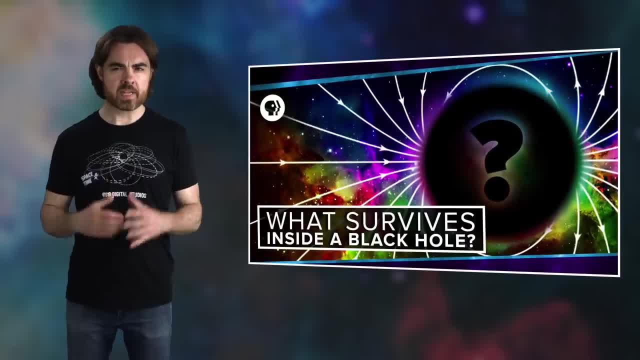 trace the universe backwards and forwards in time. The second idea was the no-hair theorem. It states that black holes can only exhibit three elements: mass, electric charge and angular momentum. The inescapable event horizon shields the outside universe from any other influence within the black hole. 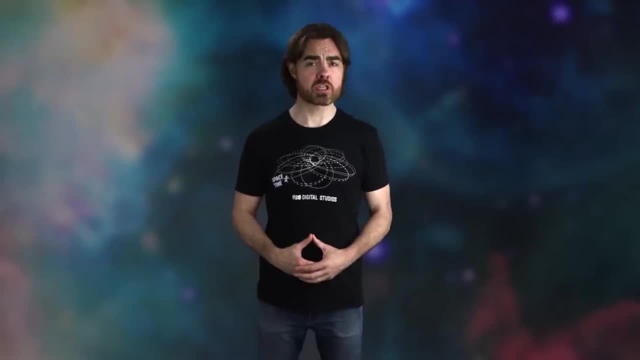 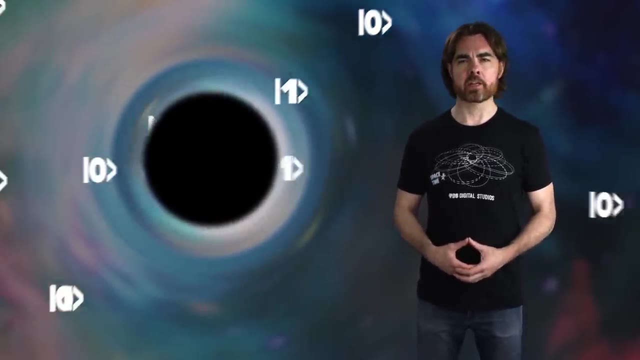 At first glance the no-hair theorem seems to contradict the conservation of information. If we see a black hole, how can we possibly figure out what particles went in to form it? But actually, by itself the no-hair theorem isn't really a problem, Because even though 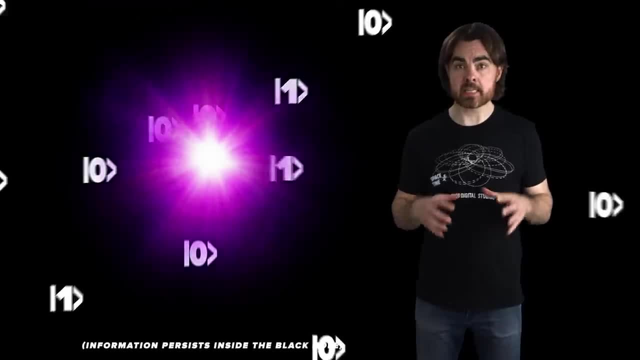 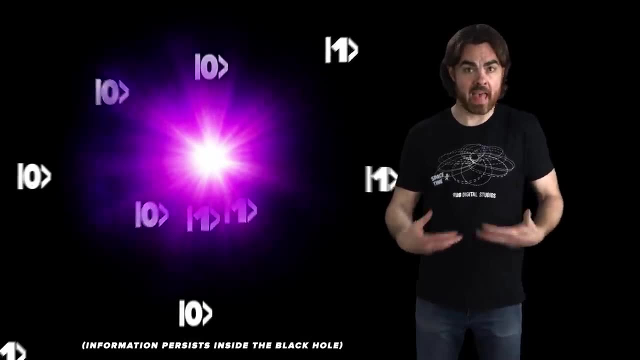 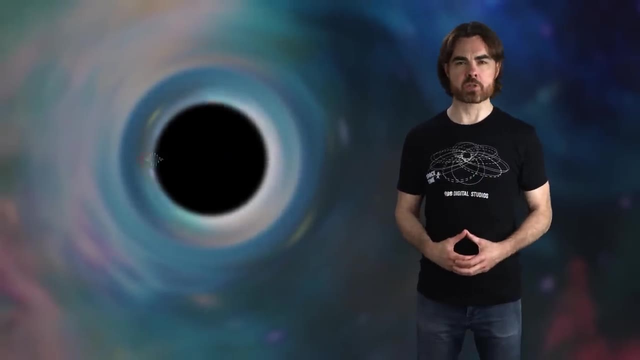 the black hole swallows information. that information persists inside the black hole. There's nothing about the law of conservation of information that requires information to remain within our accessible part of the universe. just that it continued to exist somewhere. But this is where Hawking radiation comes in. Hawking radiation is like a cosmic whiteboard. 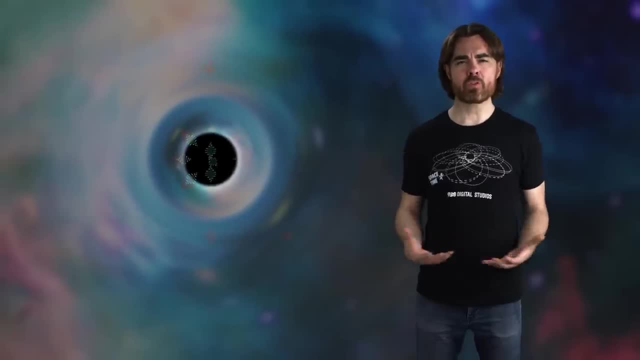 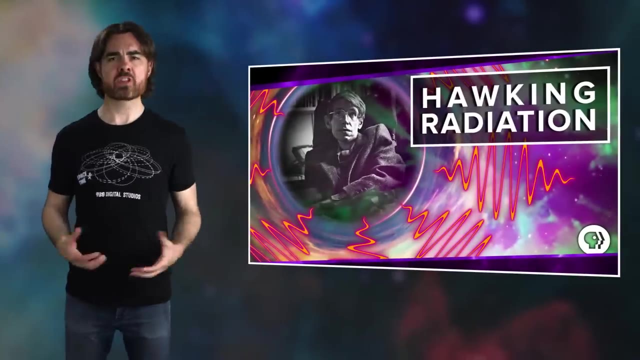 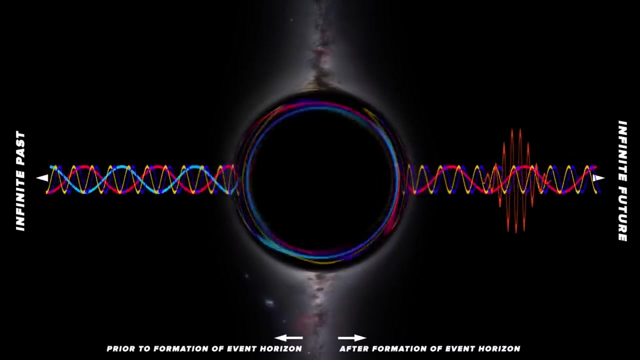 eraser. It causes black holes to evaporate into a perfectly random buzz of radiation that contains none of the information about the original contents of the black hole. We went over this in detail previously, but the TLDR- The gravitational field of a black hole- is expected to distort the surrounding quantum. 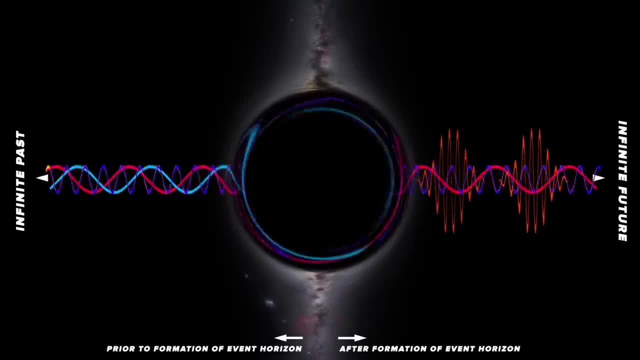 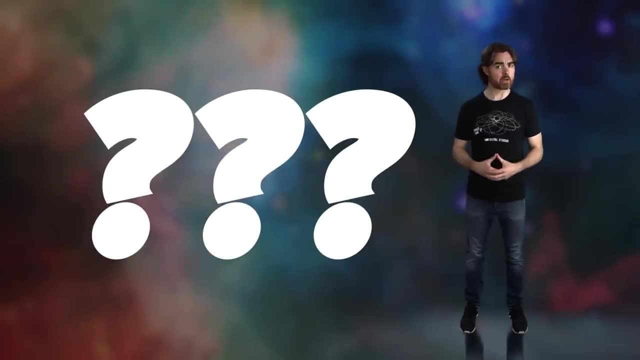 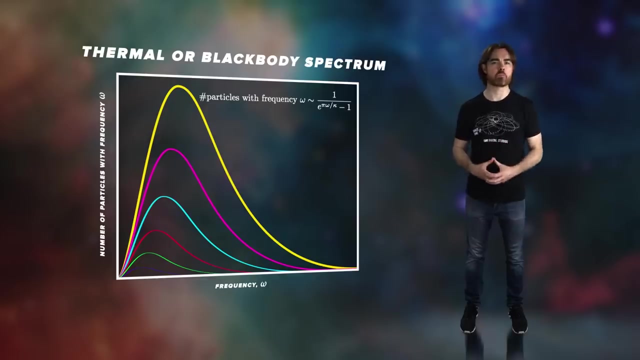 fields. That distortion looks like particles flowing away from the black hole, And the energy to create those particles must come from the mass of the black hole itself. What type of particles? According to Hawking's calculation, those particles should come out with energies that follow the black body spectrum, In other words, Hawking radiation should look. 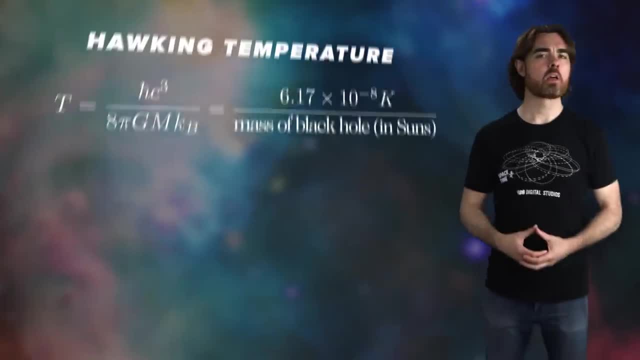 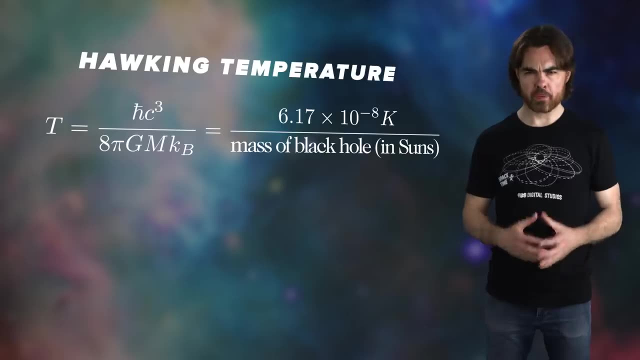 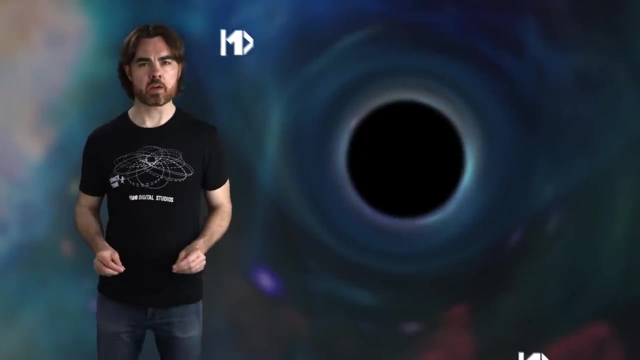 exactly like the thermal radiation of heat. So they have a temperature that is inversely proportional to their mass, And the mass of the black hole should be the only thing that determines the nature of the radiation. The key here is that Hawking radiation doesn't depend at all on what the black hole is made. 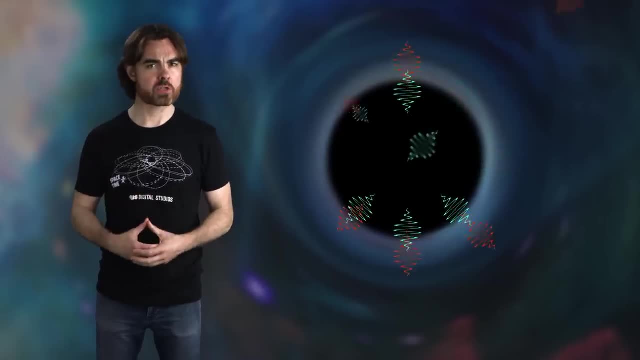 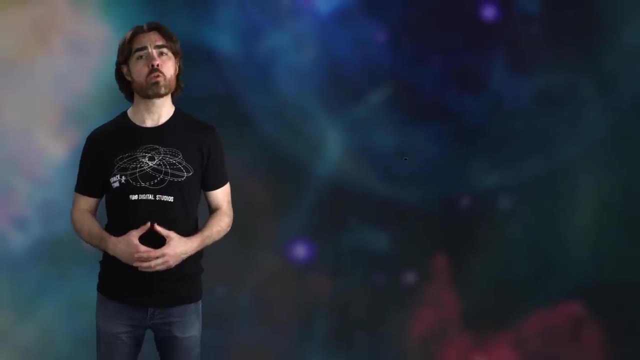 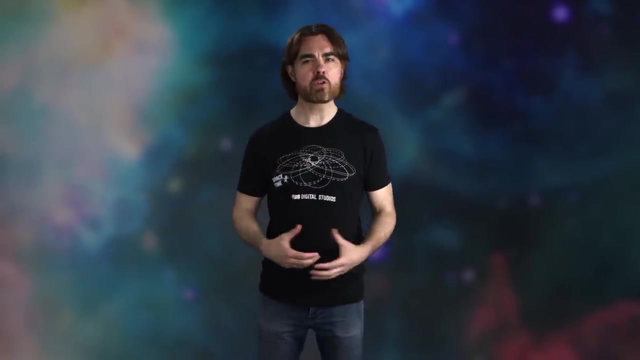 of The black hole radiates particles, mostly photons, that contain no information. Eventually, the black hole must completely evaporate into those particles, leaving no clue as to what fell into it in the first place. And that's the black hole. That's the information paradox. Through his radiation, Stephen Hawking found a way to 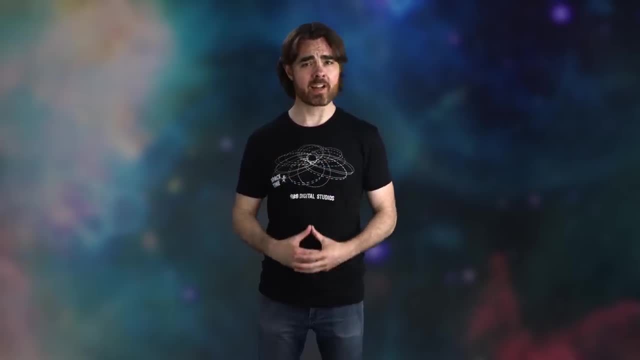 erase quantum information, which is in severe violation of one of the foundational tenets of quantum theory. And when Hawking first pointed out the paradox in the mid-70s, physicists were skeptical that there was a real problem. After all, without a theory of quantum gravity, Hawking 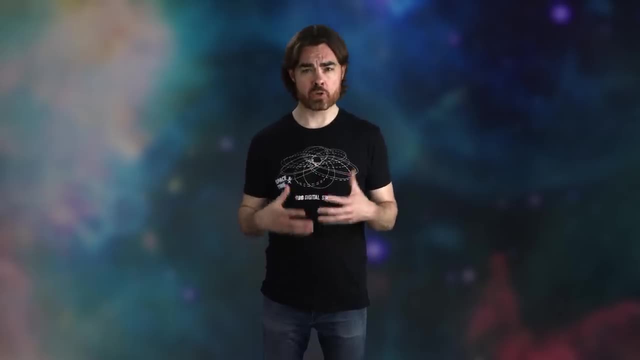 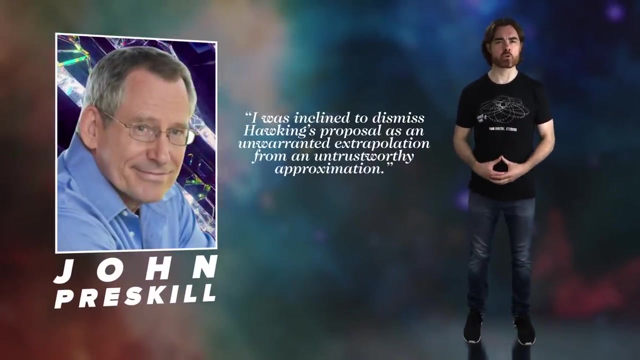 had to hack both general relativity and quantum field theory to do the calculation, To quote theoretical physicist John Preskill. I was inclined to dismiss Hawking's proposal as an unwarranted extrapolation from an untrustworthy approximation. But over time the importance. 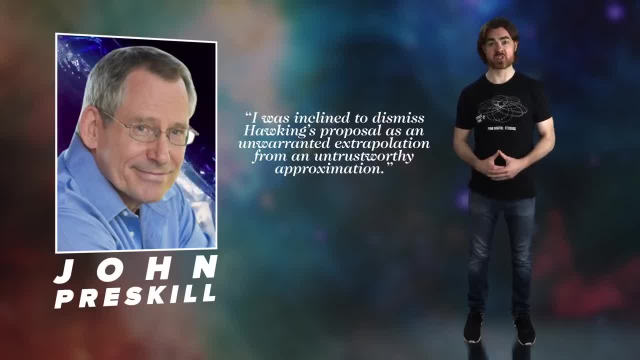 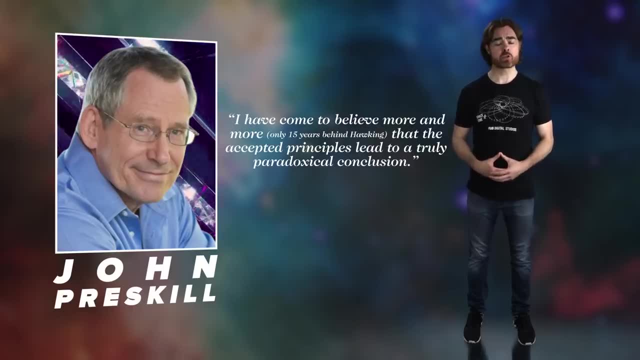 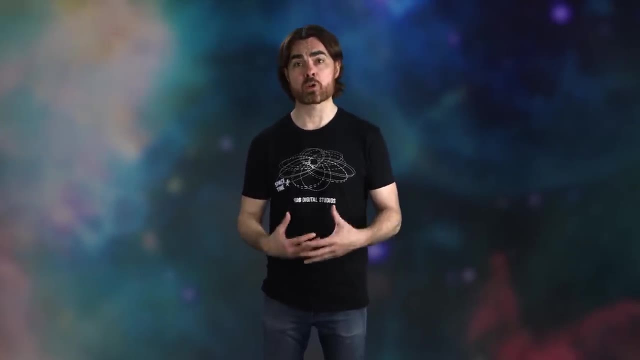 of the contradiction became clear. Preskill went on to say: I have come to believe more and more, only 15 years behind Hawking, that the accepted principles lead to a truly paradoxical conclusion. So it turns out that if we assume that both general relativity and quantum field 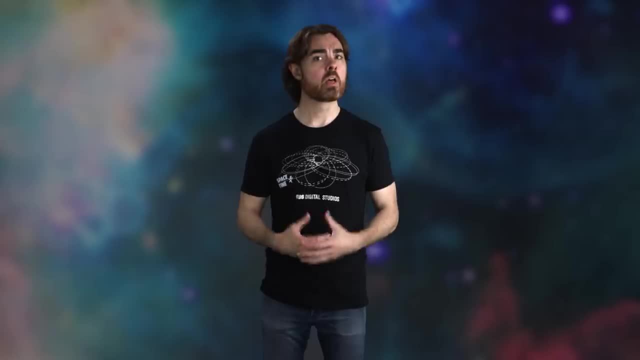 quantum field theory are correct as we currently understand them, then Hawking radiation must exist and it must erase quantum information, But there's no such thing as a true paradox. A deeper understanding of general relativity or of quantum field theory must resolve this. 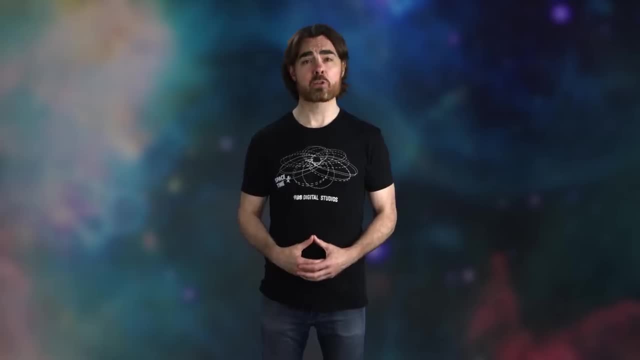 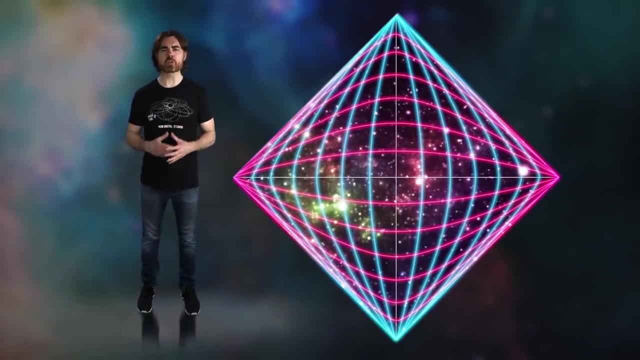 The search for the resolution to this paradox has led to some incredible new physics and some pretty astounding ideas. One of the early solutions is the most outlandish but was strongly supported by Hawking Under a slight modification of general relativity called Einstein-Cartan theory. it's predicted 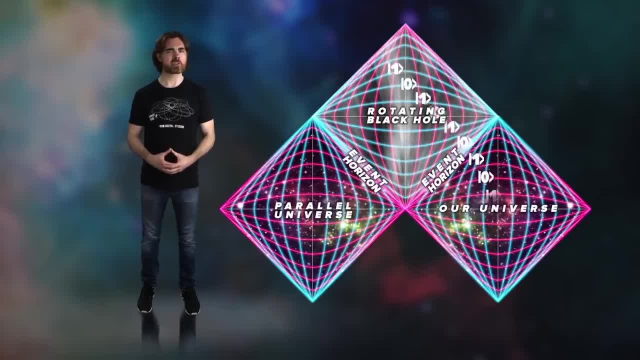 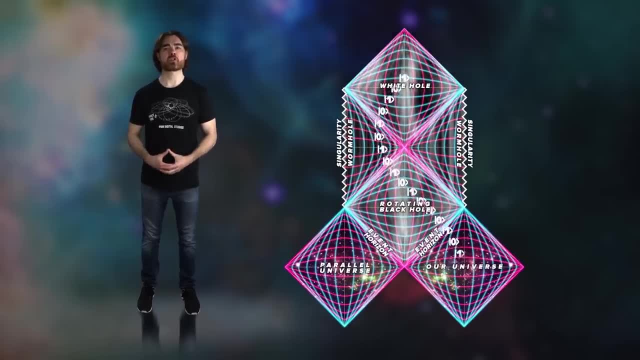 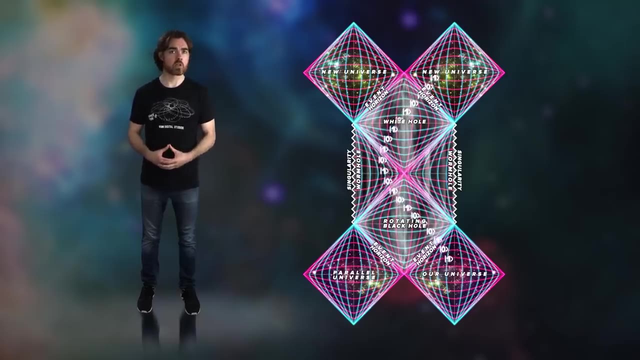 that the formation of a rotating black hole gives birth to an entire new universe accessible by a wormhole. That's cool. so what if all of the information lost into the black hole ends up in the new universe? It would be forever inaccessible to us, but would still exist. 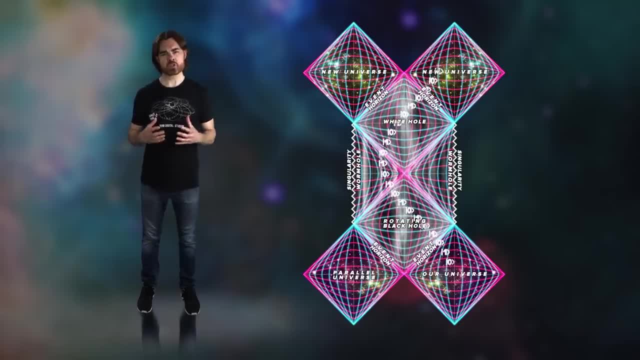 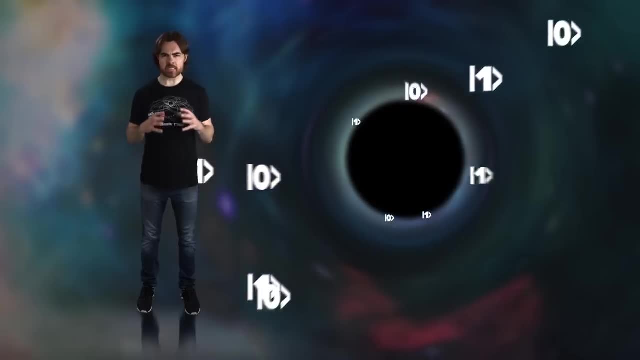 This solution to the paradox has been attributed to Freeman Dyson, but was championed by Hawking for many years. The competing idea is that the information of everything that falls into the black hole becomes imprinted on the Hawking radiation itself, so it stays in this universe. 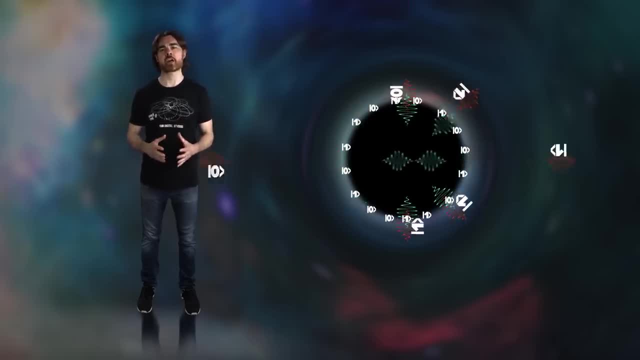 No new universe is required. A motivation for this idea is the fact that, from the point of view of an outside observer, nothing ever actually crosses the event horizon For the outside universe. everything that ever fell into the black hole remains frozen in time and smeared flat over that horizon. 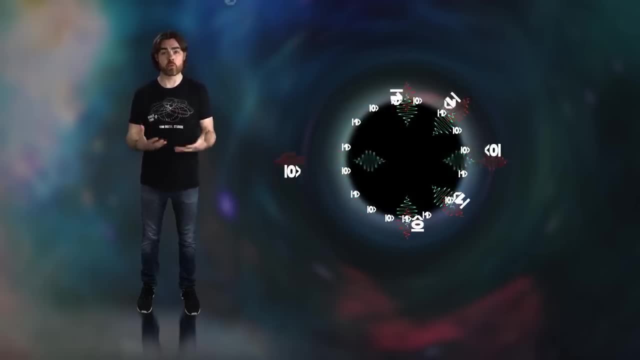 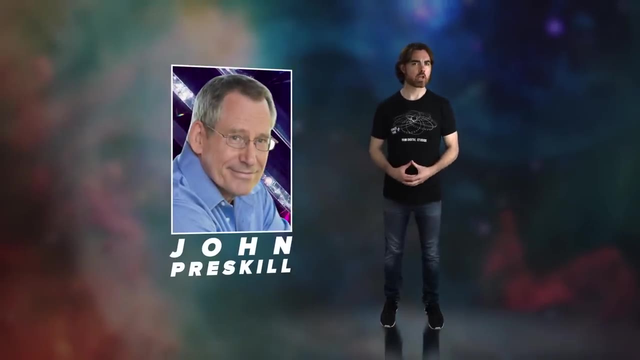 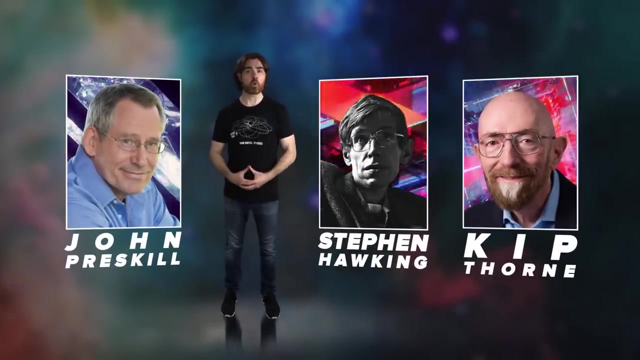 It's essentially invisible, but in principle the information is still there. In 1997, the debate between these ideas became a bet. On one side, John Preskill bet that information somehow leaked back out into the universe. On the other side, Stephen Hawking and Kip Thorne bet that it was forever lost from our 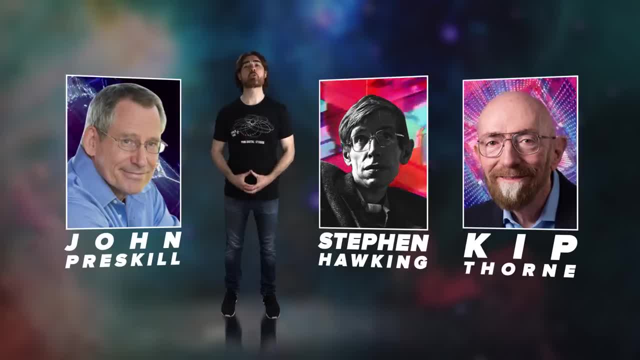 universe And the stakes: An encyclopedia of the winner's choice from which information can be retrieved at will. To resolve the bet, physicists and scientists from the University of New York, the University of New York and the University of New York have come up with an idea. 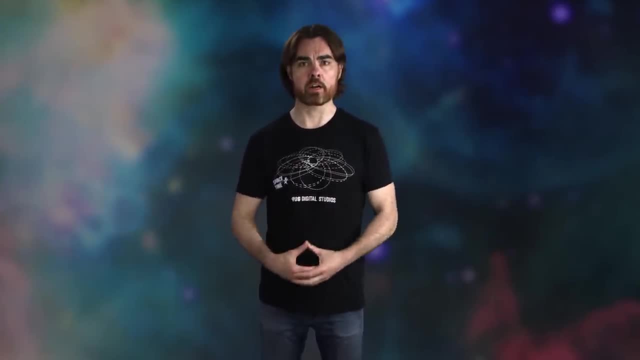 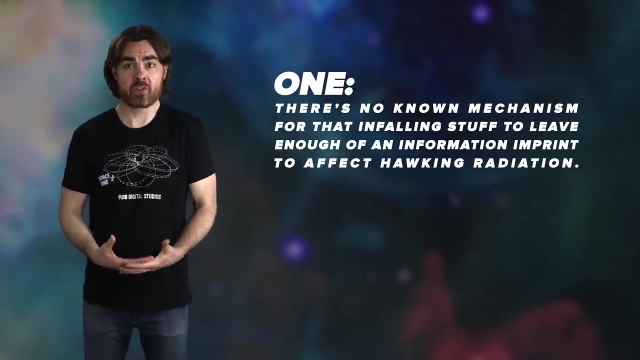 Scientists had to figure out how quantum information could be transferred to Hawking radiation. But there are two gigantic problems with this idea. One: there's no known mechanism for that in-falling stuff to leave enough of an information imprint to affect Hawking radiation. 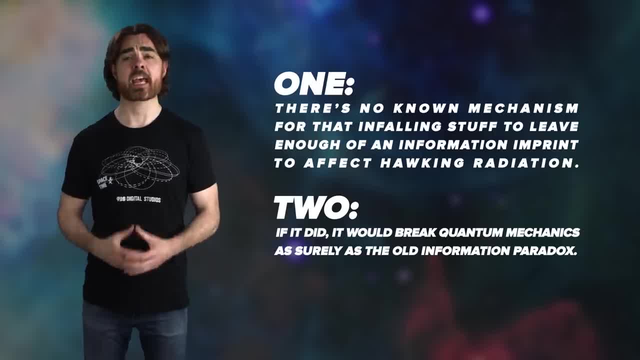 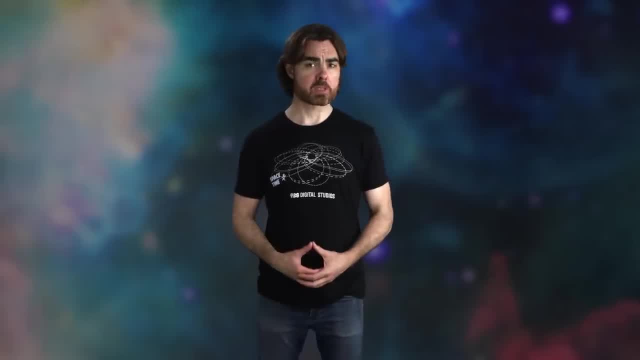 And two: if it did, it would break quantum mechanics as surely as the old information paradox. Let's start with the second point. It turns out that by transferring quantum information to Hawking radiation, you may still violate the law of conservation. 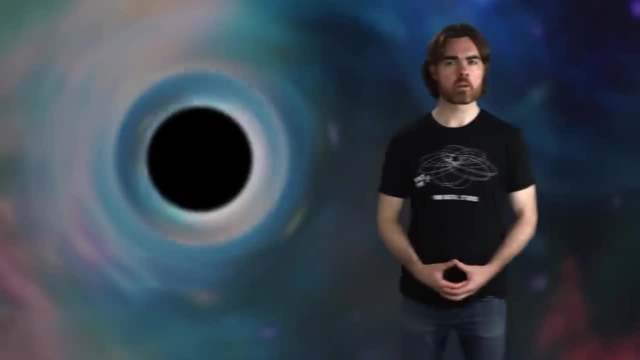 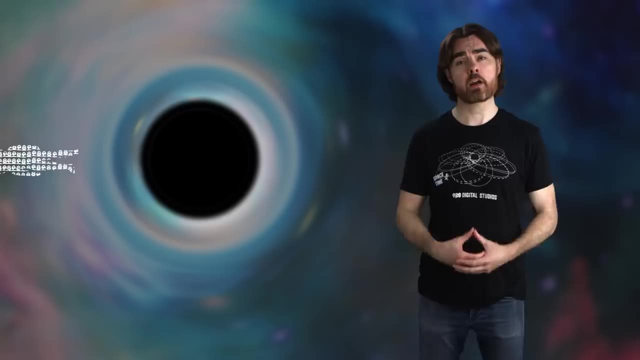 The law of conservation is the law of conservation of information just as much as you would by deleting it From the point of view of an observer falling into the black hole. they aren't frozen at the horizon, They fall straight through, carrying their information with them. 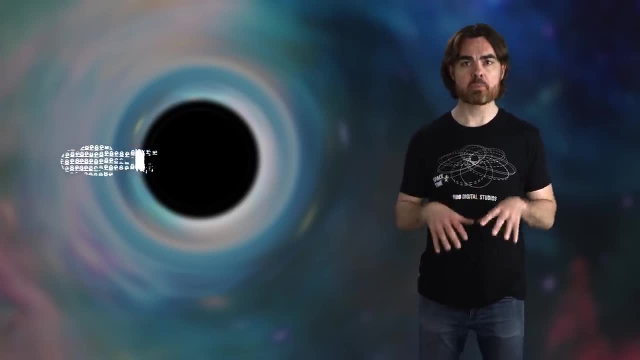 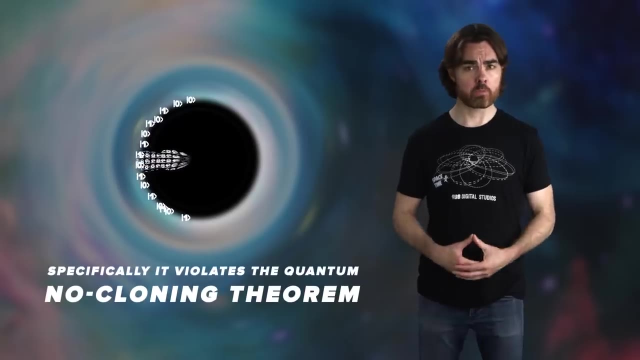 That means their information would radiate back out into the universe and be absorbed into the black hole. The information would be duplicated, violating conservation of information. Specifically, it would violate the quantum no-cloning theorem. Physicist Leonard Susskind has argued that there is no violation. 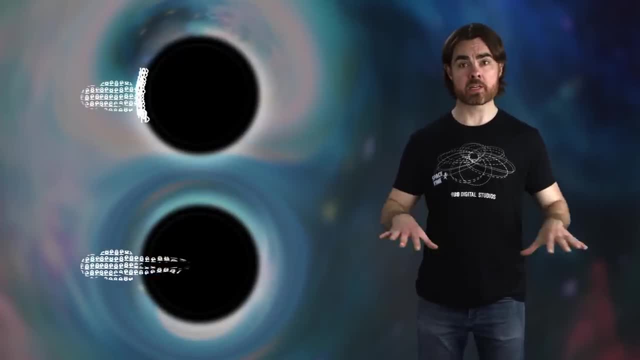 The two copies of the information are completely disconnected. No observer can ever see both. In fact, because the interior of the black hole doesn't even exist on the same timeline as the external universe, it's arguable that those copies don't even exist at the 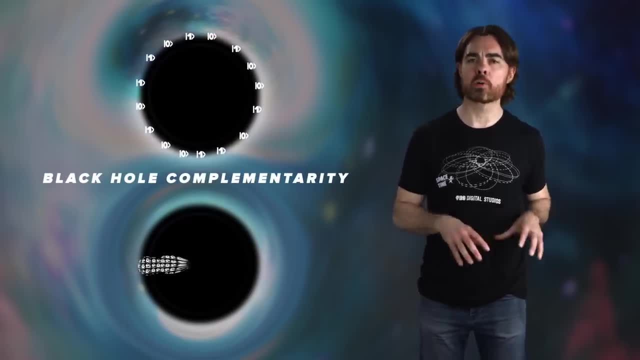 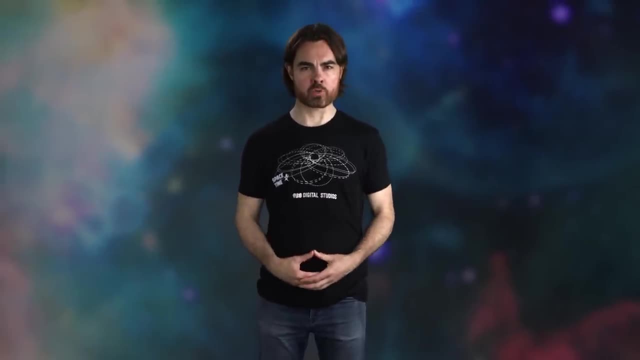 same time. This idea is known as black hole complementarity. You might remember that there are certain pairs of quantum observable, complementary observables, like position and momentum, that can't both be perfectly balanced and can't be measured at the same time. 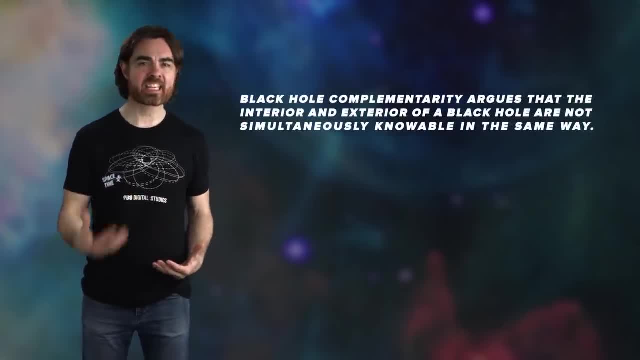 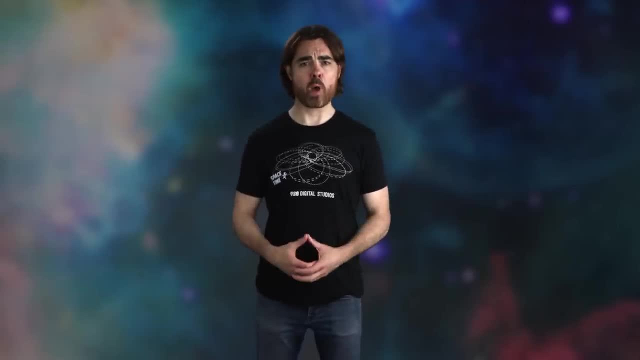 Black hole complementarity argues that the interior and exterior of a black hole are not simultaneously knowable in exactly the same way. OK, so we can argue our way around the no-cloning theorem with black hole complementarity, But there was still no known mechanism for this to happen. 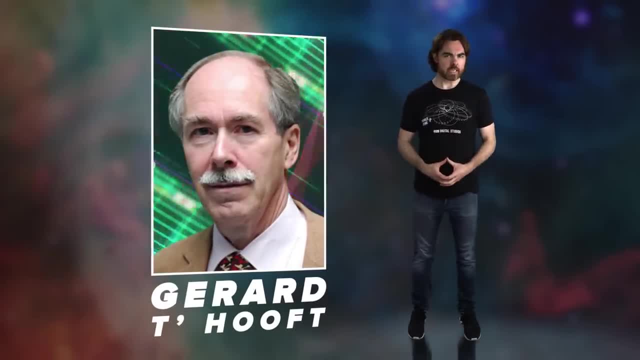 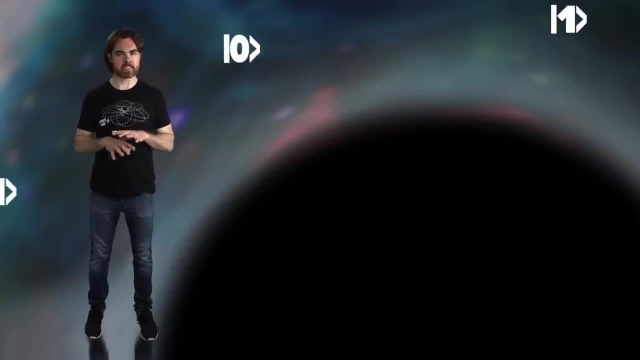 The solution began with physicist Gerard Etouft. He did a more careful calculation of the effect of infalling material and found that it doesn't exactly freeze above a completely static horizon. rather, it distorts the horizon, creating a sort of lump at the point of crossing. 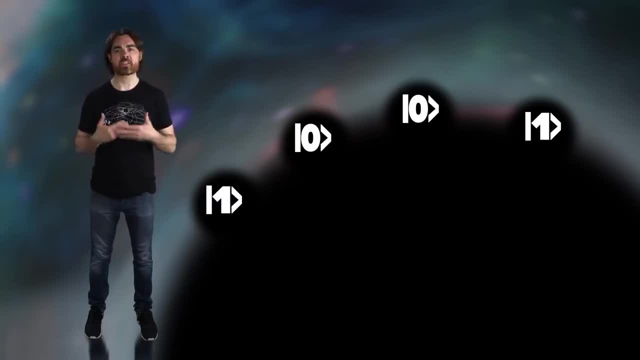 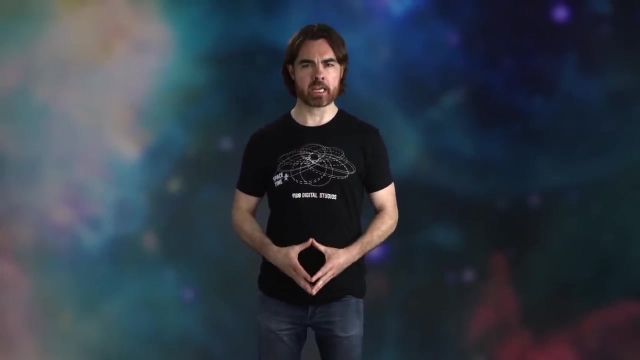 Those distortions should contain all of the information about the infalling material And, in principle, those distortions could potentially influence outgoing Hawking radiation, allowing them to carry away their information. This idea seems straightforward, but it has stunning implications. Etouft realized that the three-dimensional gravitational equation of black hole complementarity 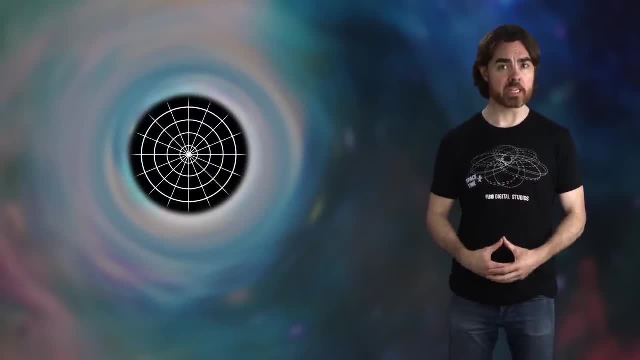 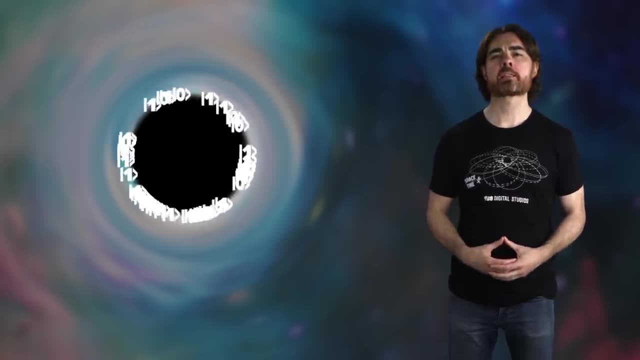 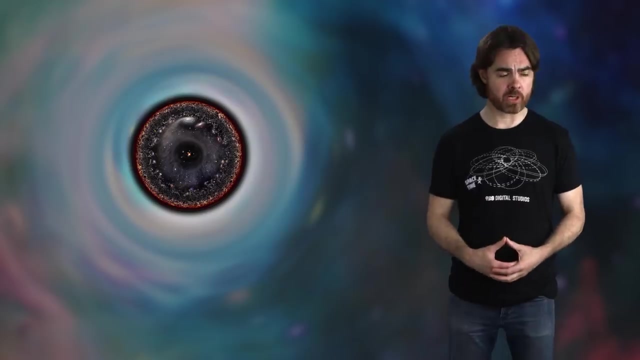 could be fully described by interactions on a 2D surface that did not include gravity. This led him to realize that the union of quantum mechanics and gravity may require that the entire 3D universe be a projection on a 2D structure. Leonard Susskind formalized this idea in the context of string theory in what we now know. 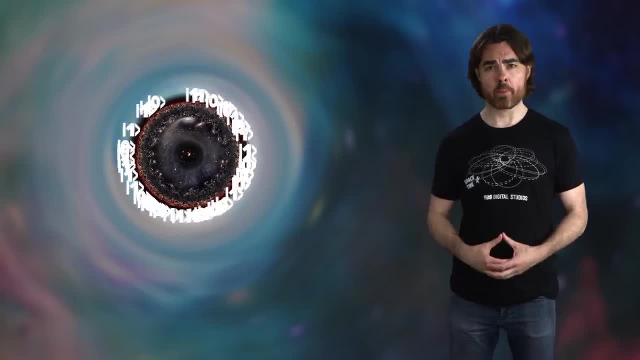 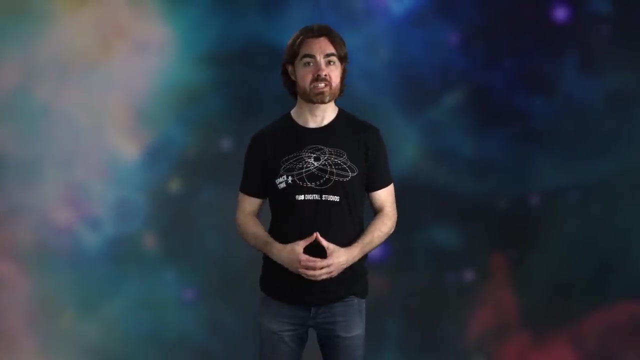 as the holographic principle. This is definitely something we'll come back to, Because, besides giving a concrete mechanism by which information can be stored on the surface of a black hole, it may imply that the entire universe is a hologram. Exactly how the information on an event horizon gets attached to Hawking radiation is still. 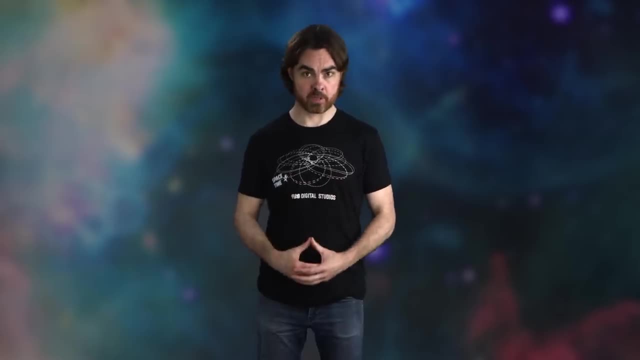 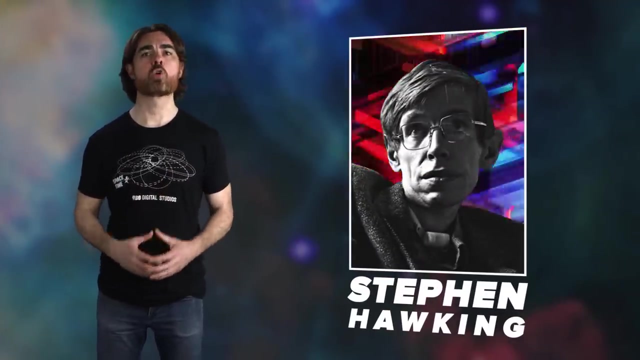 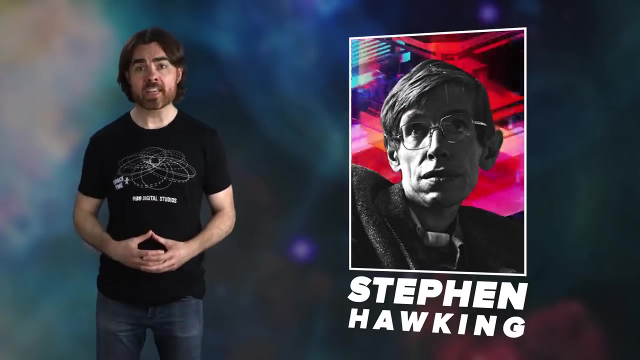 contentious, but a number of physicists have proposed possibilities. Stephen Hawking himself has also jumped into that game, suggesting that quantum tunneling from within the black hole could interact with the holographic horizon and carry information out into the universe. But to enter the game, Hawking had to concede the old bet and admit that information does. 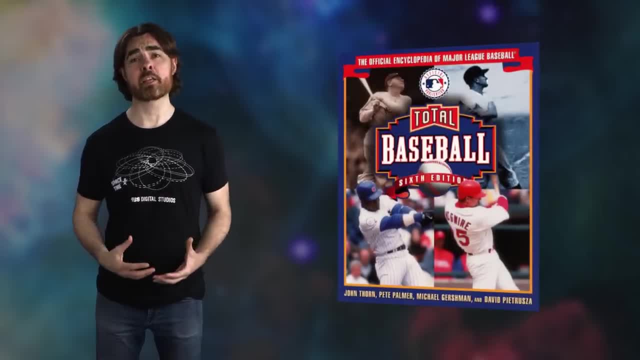 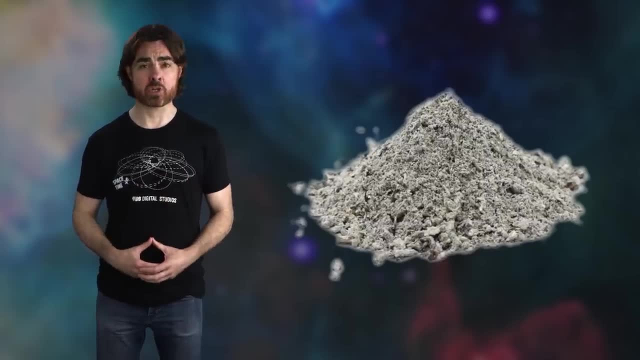 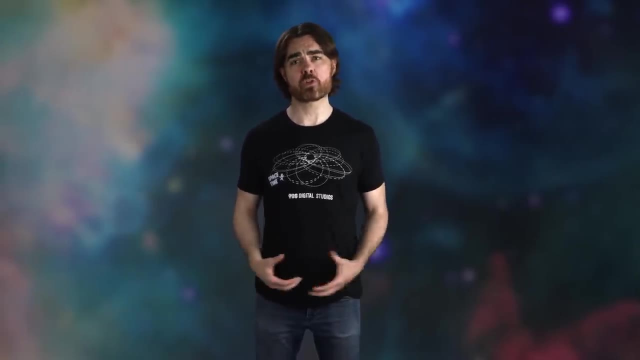 escape black holes. He gave John Preskill an encyclopedia of baseball but joked that maybe he should have given him the ashes of one to better reflect the scrambled information in Hawking radiation. The idea of black hole complementarity and the results it led to are by no means fully. 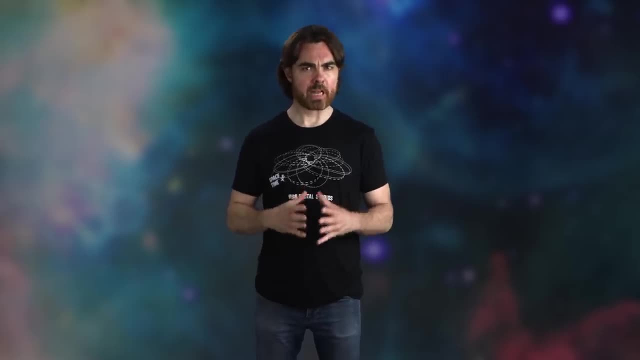 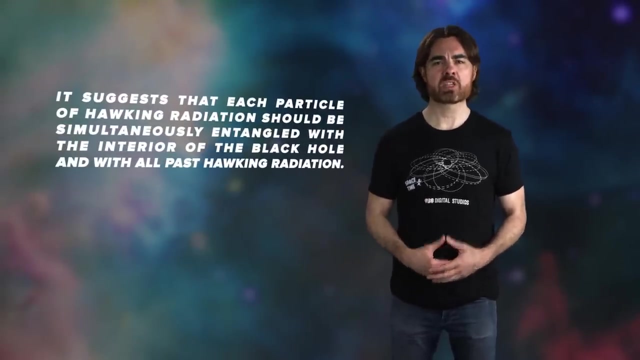 accepted. They are of course untested. But black hole complementarity introduces the idea that black hole complementarity is a black hole. It suggests that each particle of Hawking radiation should be simultaneously entangled with the interior of the black hole and with all past Hawking radiation. 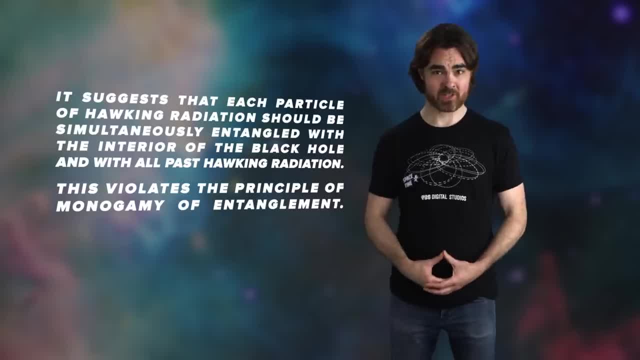 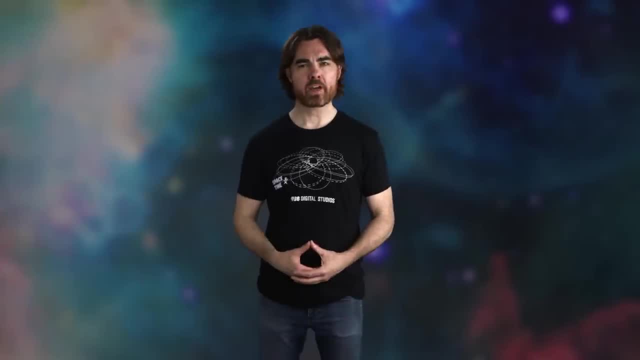 This violates the principle of monogamy of entanglement. We'll have to come back to this also and to the proposed solution, the black hole firewall. It never fails to amaze me how one little loose thread, a seemingly insignificant quirk. 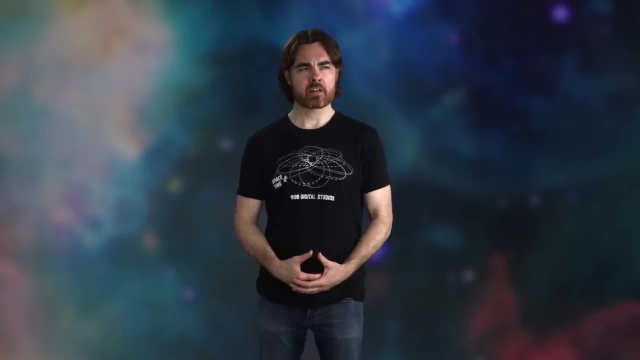 in the theory can lead to massive discoveries. But it's not all that simple. It has been the basis of many discoveries and complete reframings of physics- That cute little 1974 paper in which the young Stephen Hawking showed that black holes must. 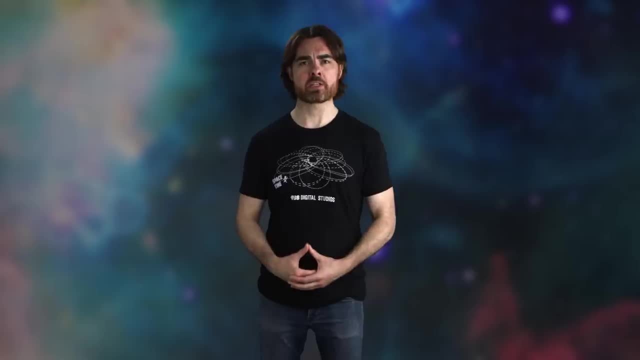 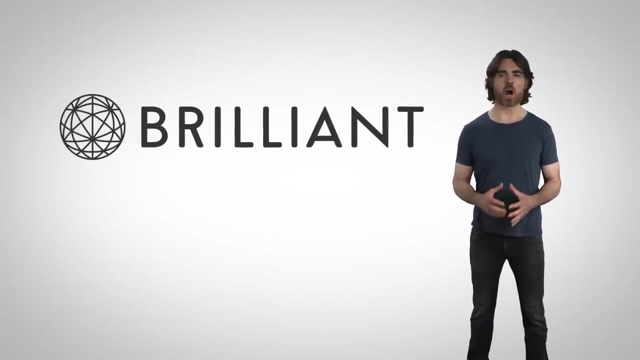 leak very slightly has led to radical new ideas about the nature of information and entropy, exploded the field of string theory and hinted at the possible holographic nature of spacetime. Black holes represent the ultimate victory of gravity. Einstein's general theory of relativity reveals them to be regions of frozen time-and-space. 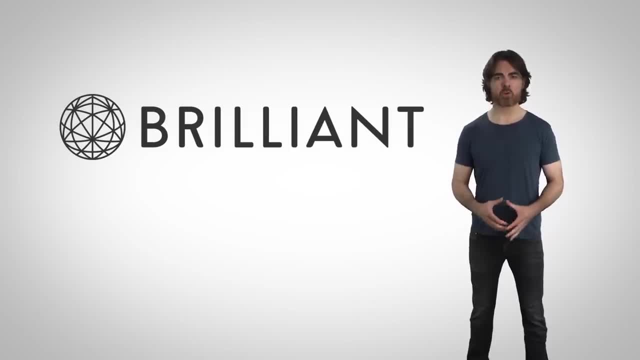 They are more than just black holes and time and cascading space. But the first hint of the existence of black holes appeared long before Einstein. They were glimpsed as dark stars in the mathematics of Isaac Newton's law of universal gravitation. So to continue your own mathematical journey. 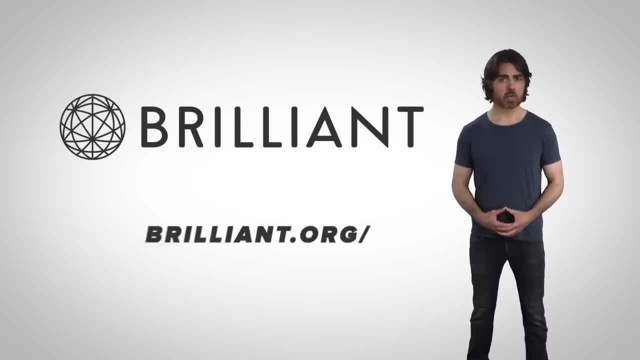 into black holes. Newton's gravity is the place to start. Brilliantorg has a really comprehensive series on gravitational physics that will take you from Newton's law all the way through gravitational field and celestial mechanics, And Brilliant leads you on this journey in a series of clear, very gettable steps. 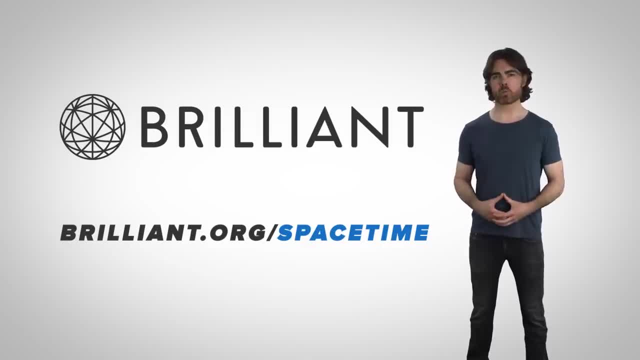 You'll be solving increasingly complex problems along the way to really training your brain to think like a physicist. Learning about physics is much more than facts and memorizing, But when done right, it can give you a whole new way to look at the universe itself. 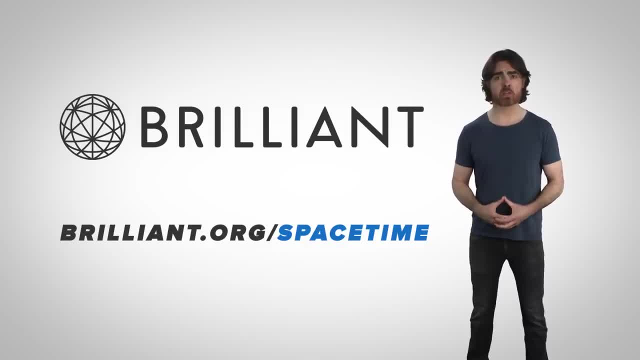 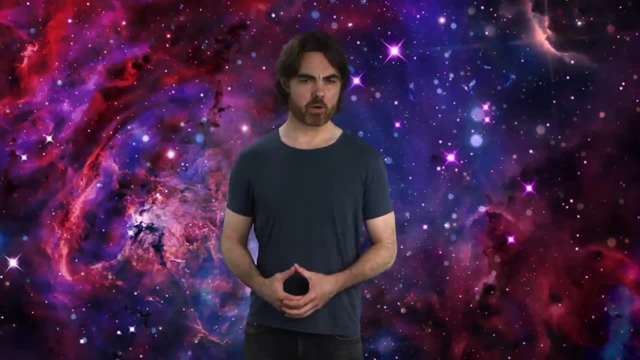 Brilliant math and science done right is proud to support Space Time. To learn more about Brilliant, go to brilliantorg slash spacetime. Last week we talked about the no hair theorem of black holes And you all had some hairy questions. 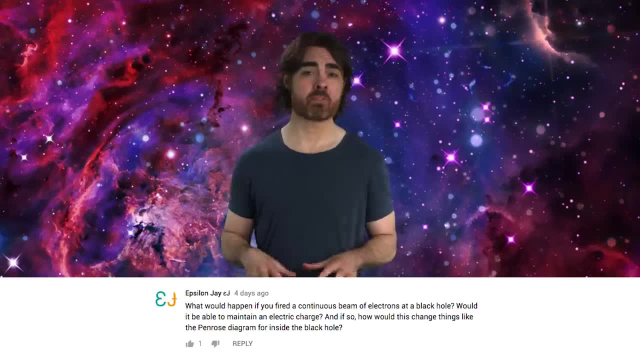 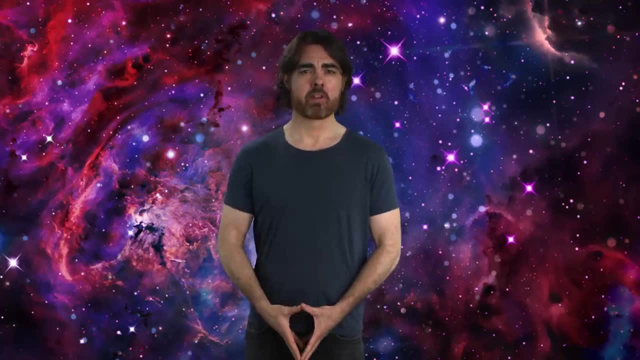 Epsilon J asks what would happen if you fired a continuous beam of electrons at a black hole, And how would the charge affect the Penrose diagram? Great question: If you keep injecting charge into a black hole, then it does maintain an electric charge. 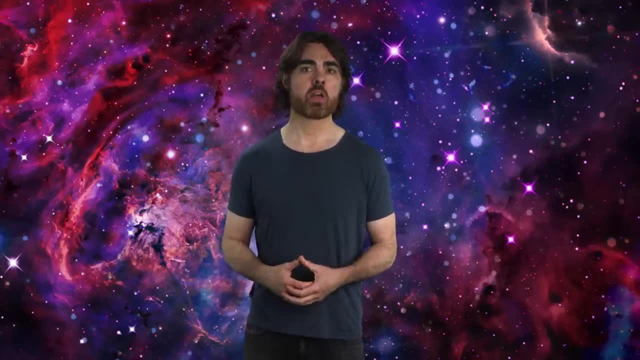 That charge only decays if the black hole is left to its own devices. And it turns out that a charged black hole has a pretty weird Penrose diagram. The exterior looks pretty weird. It's pretty similar to a regular black hole, but the inside is very different. 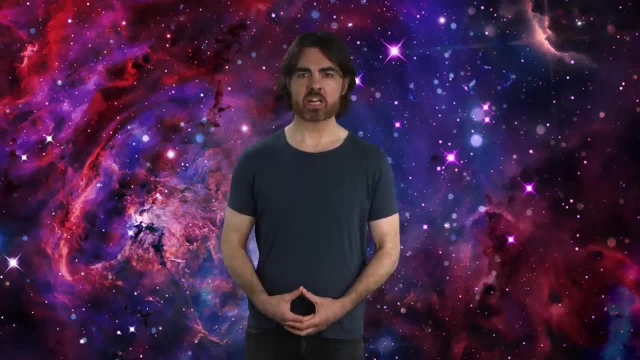 The electric charge within the black hole produces a negative pressure that actually halts the cascade of space within the black hole and propels it back outwards. In the mathematics it looks as though anything falling into a charged black hole is ejected into a separate universe. 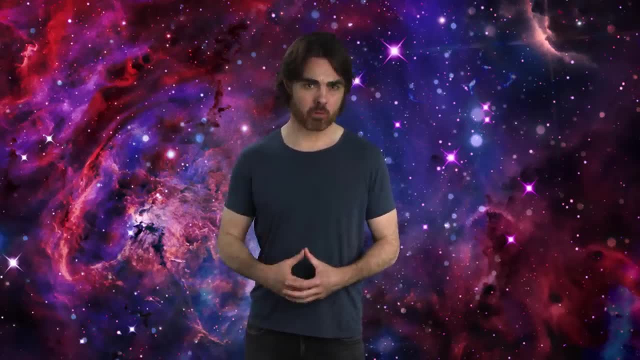 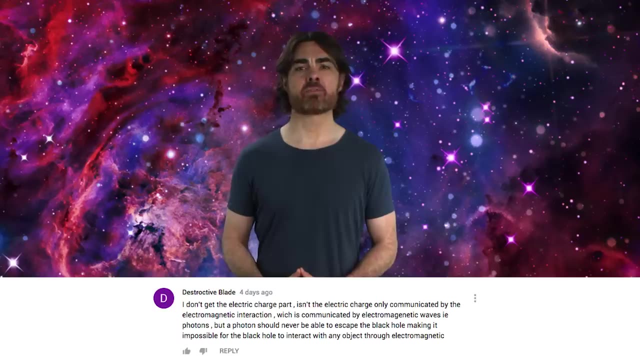 That's a universe of weirdness that we'll do an episode on at some point. Destructive Blade asks how it can be that the outside of a black hole can feel its electric charge, given that the electromagnetic field is communicated by photons and photons can't escape the black hole. 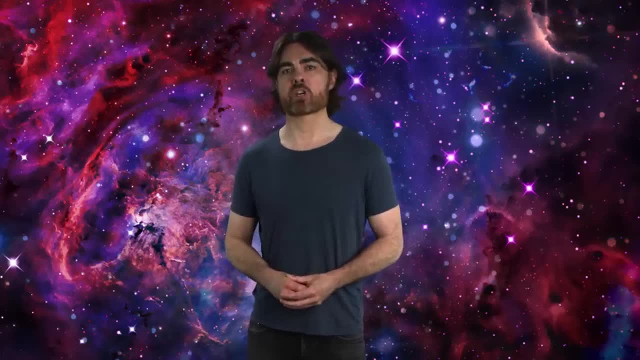 Good observation. So we talked about a black hole's electric charge in terms of the classical electromagnetic field, which has an existence independent of electric charge, But quantum field theory imagines the electromagnetic force as being transmitted by virtual photons. It's important to note the distinction. 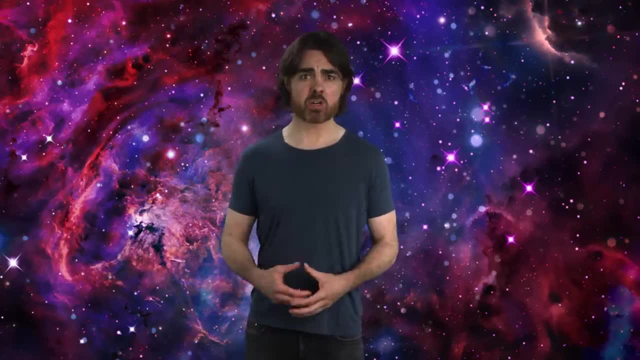 between virtual photons and real photons. Virtual particles in general are just a way to mathematically account for the infinite ways a quantum field can communicate its influence. Virtual particles don't have the same restrictions as regular particles. They can have any mass can travel faster than light. 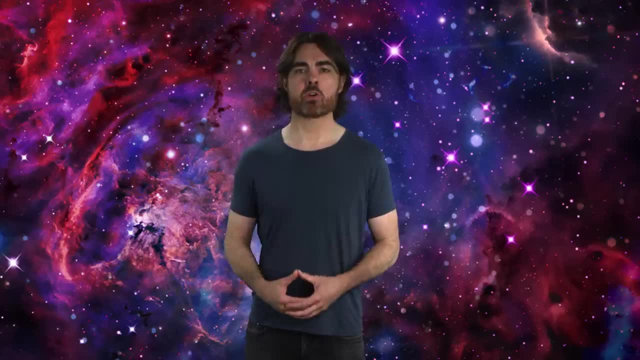 and can even travel backwards in time. Check out our episode on the path integral and Feynman diagrams for more info on this wackiness. In this picture, virtual particles can escape a black hole to communicate the influence of the charge within, But it's important not to take the existence of these particles. 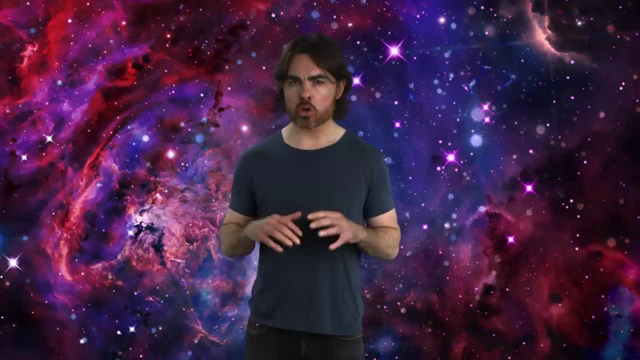 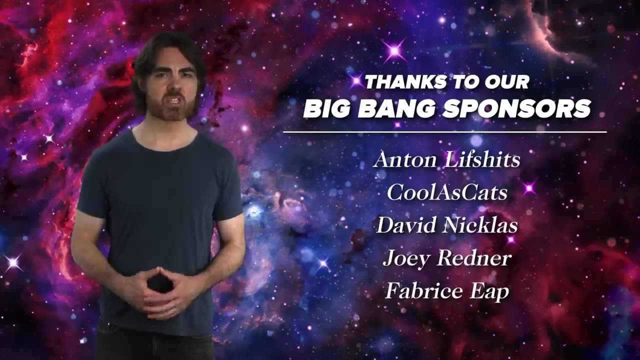 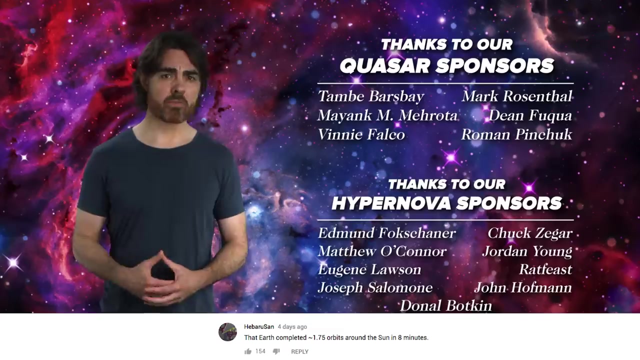 too seriously. The electromagnetic field outside the black hole knows about the charge inside the black hole, But whether that's because of virtual particle interaction with the interior or just the persistence of the field at the event horizon is a matter of interpretation. Hirabu-san noticed that in our graphic. 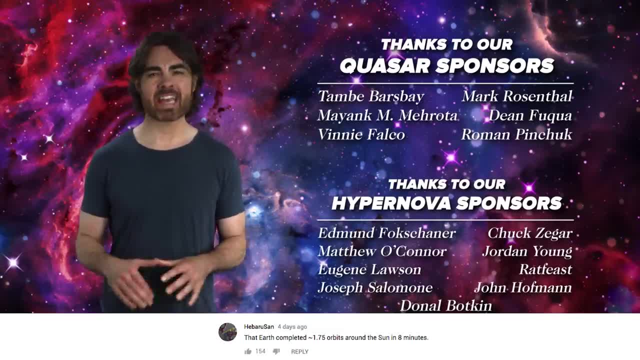 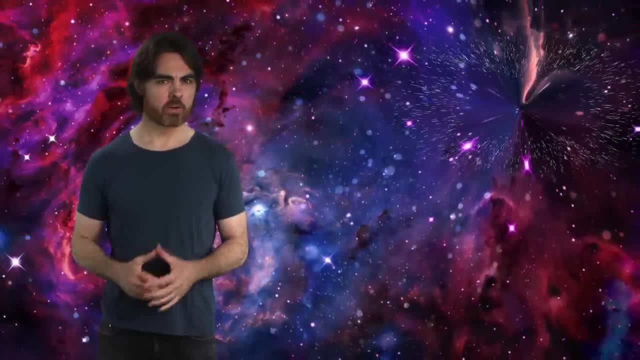 the Earth completed 1.75 orbits in the supposed eight minutes it took the sun's gravitational field to vanish. Yeah, that was due to time dilation. There's a very certain special frame of reference, like when you're trying to throw together a quick graphic.